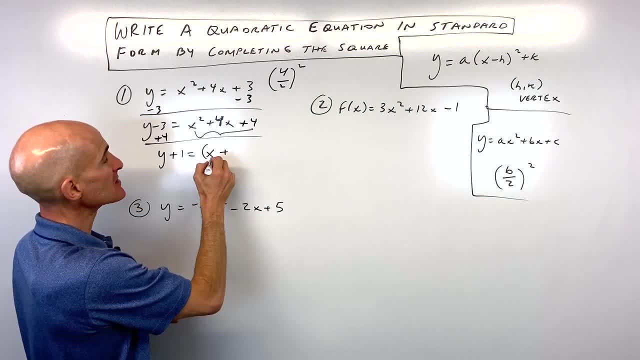 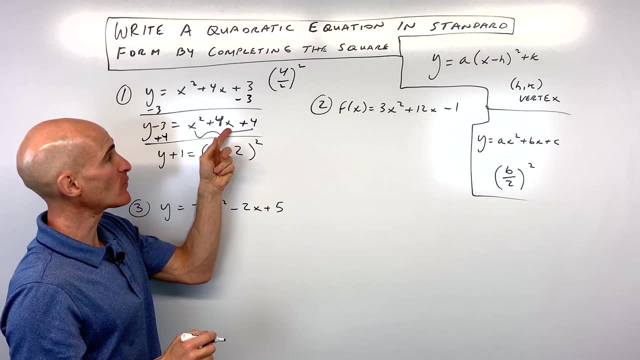 write this as a binomial squared, So it's going to be x plus 2, the quantity squared. It's always going to be half of this b value. so if this was minus 4x, I would write minus 2 here. Okay, we're almost there. 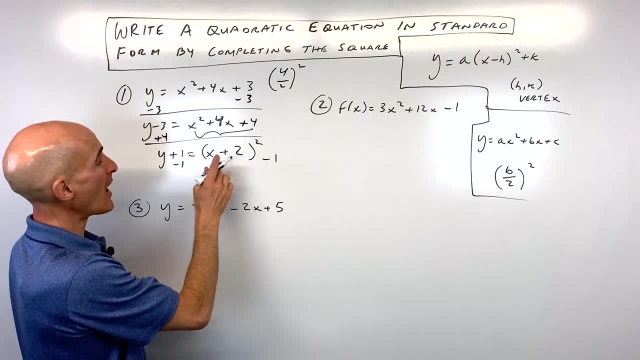 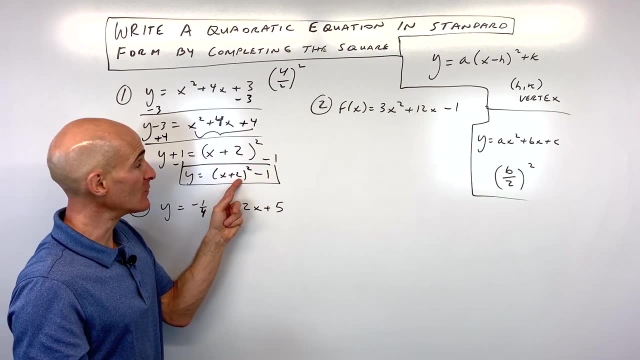 now the last thing is I'm going to subtract 1, because what I want to do is I want to get y by itself. so y equals x plus 2 squared minus 1, and you can see the vertex is going to be negative, 2 negative 1.. Remember, the one group with the x is going to have the opposite sign, because this is x. 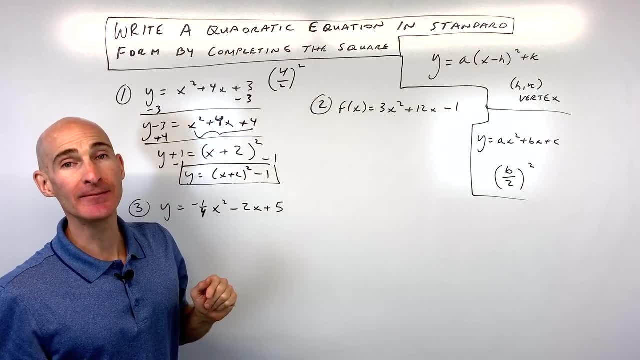 minus h. So vertex negative 2, negative 1, and you got it. So for number two, now a little bit more challenge here, and what we want to do is we want to find the second sign. So we want to find the first word, so we want to find the second sign and we want to find the second word, because the first word 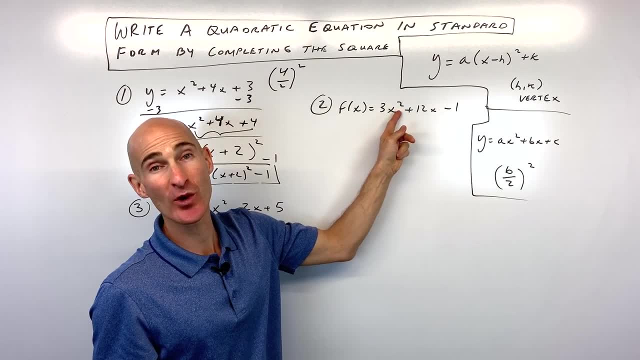 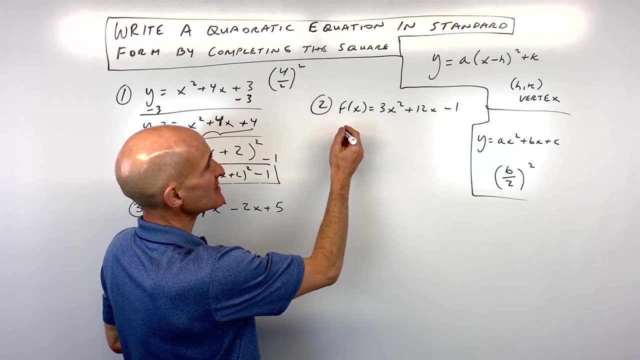 What makes this more challenging is that we have a coefficient, a number, in front of the x squared term, So our a value is not 1, it's 3 in this case. Same process, though. What we want to do is think of f, of x, as like y, and what I'm going to do is I'm going to. 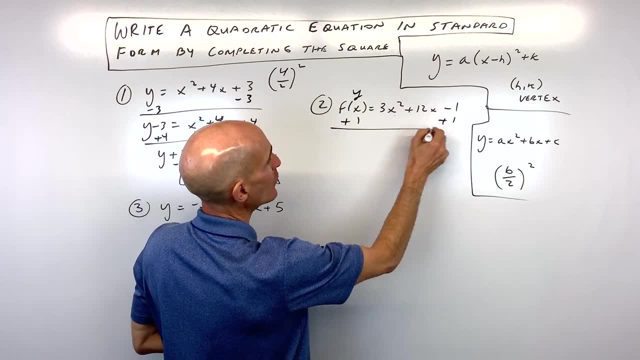 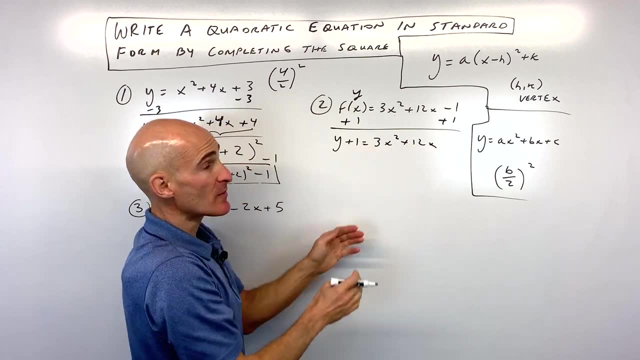 move the constant, the number, to the other side by doing the opposite: adding 1.. So that gives us: y plus 1 equals 3x squared plus 12x. What I'm going to do is I'm going to factor out that coefficient, the 3.. 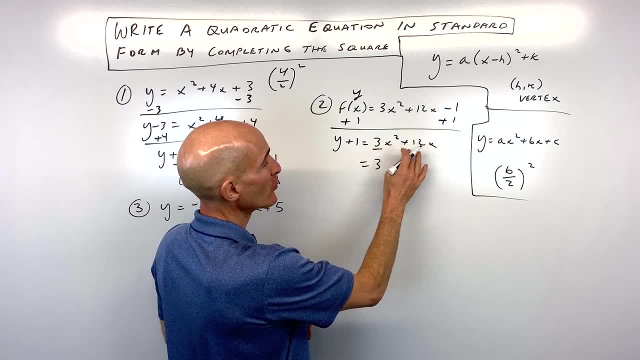 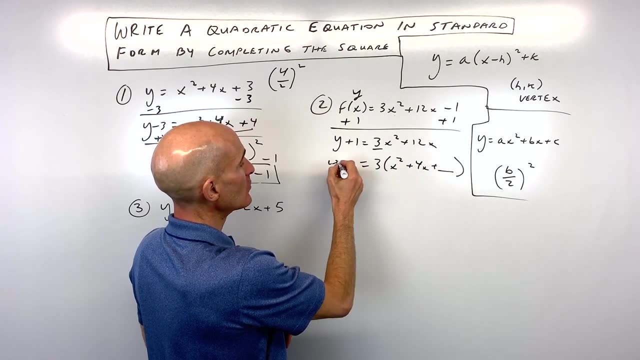 We're not taking the greatest common factor, we're just factoring out the 3 out of both of these two terms here. So we have 3x squared plus 4x plus blank. okay, equals y plus 1.. So now what I'm going to do is I'm going to complete the square. so we're going to take 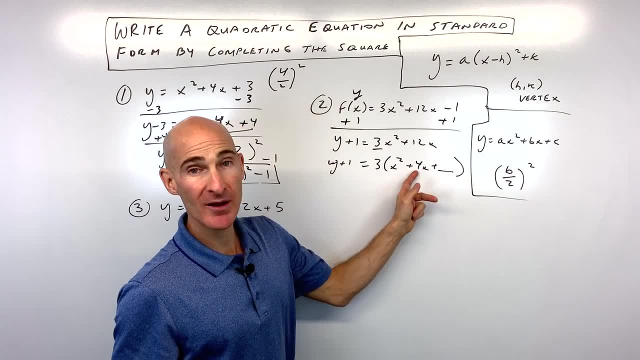 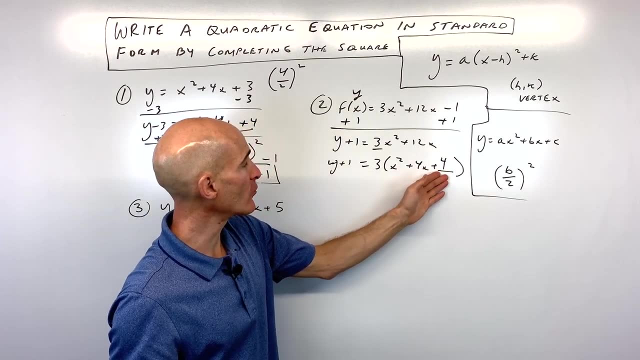 b divided by 2 and square it. So 4 divided by 2 is 2, 2 squared is 4.. Now the mistake that students make is that they say: alright, you know, Mario, I added 4 to the right, don't I add 4 to the left. 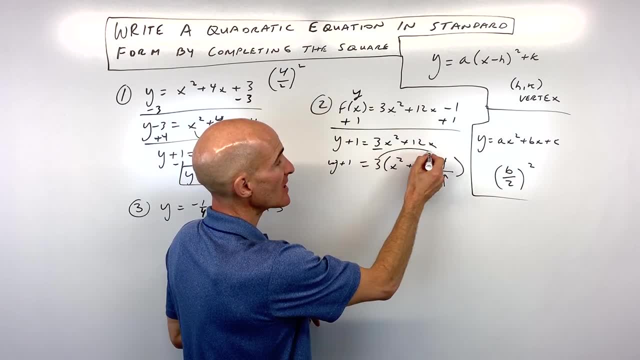 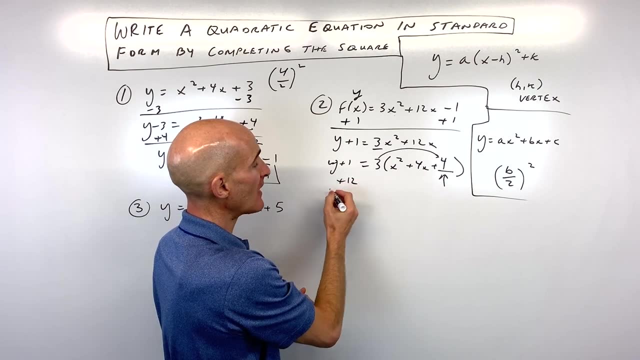 Well, the thing is to see how this 4 is inside of the parentheses. So, actually out of thin air, we're adding 3 times 4, which is 12, to the right side of the equation. To keep it balanced, we have to add 12 to the left side, okay. 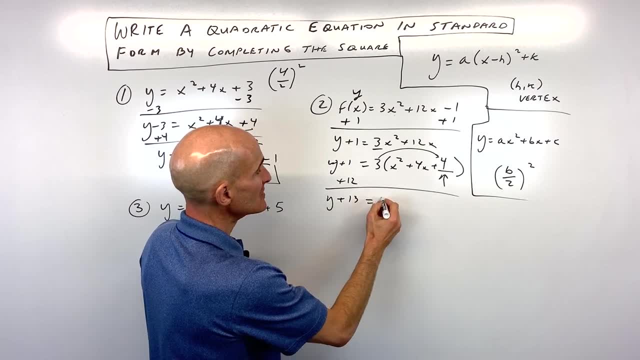 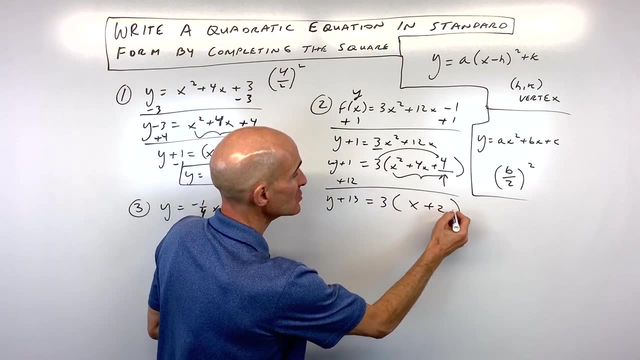 So are you with me so far? So now what we have is y plus 13 equals 3, and now what I'm going to do is I'm going to factor this quantity in the parentheses, and it's going to be x plus 2, squared very. 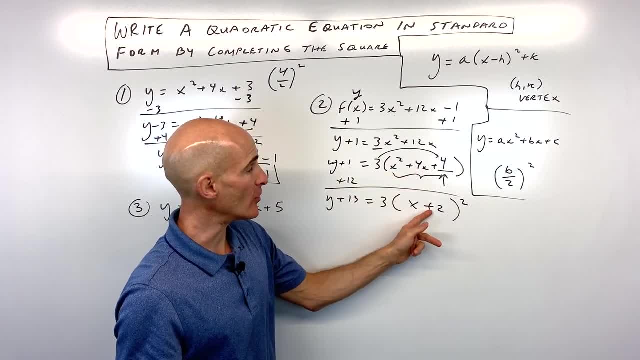 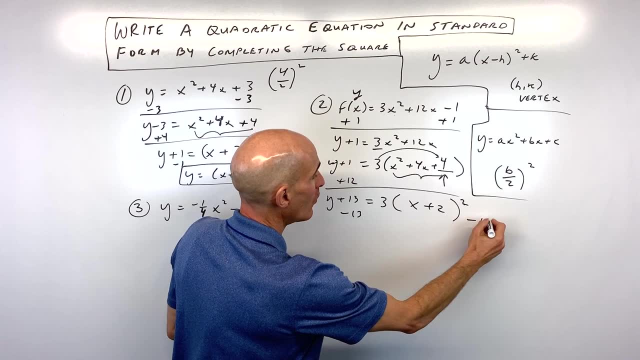 similar to this previous problem. So it's always half of that b value. If this was minus 4x, it would be minus 2.. The last thing is to move the 13 to the other side, So you get the y by itself. so you can see. our final result is 3 times x plus 2 squared. 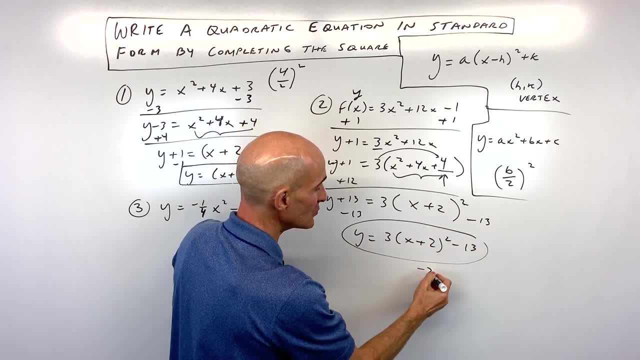 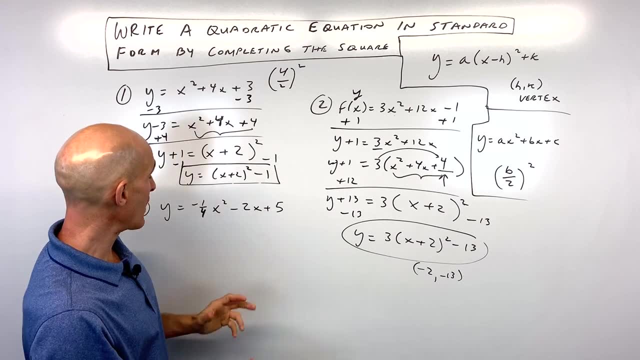 minus 13, and our vertex is going to be at negative 2, negative 13.. Remember this one- in parentheses is the opposite sign. Okay, last example: see if you can do this one. This is probably the most challenging example, because it involves a fraction as well as. 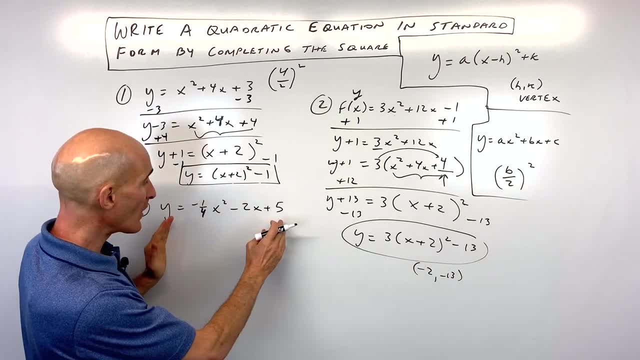 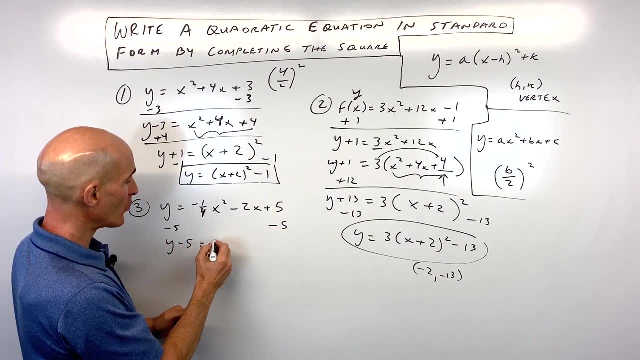 a negative. Okay, so what would you do on this one? What I'm going to do here is I'm going to subtract 5, like I normally do. okay, just to get the constant Out of the way. on the other side of the equation. 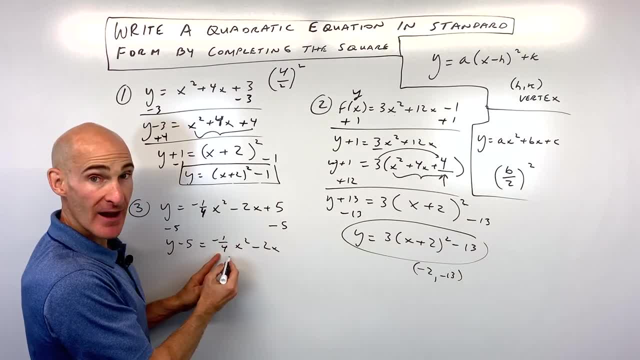 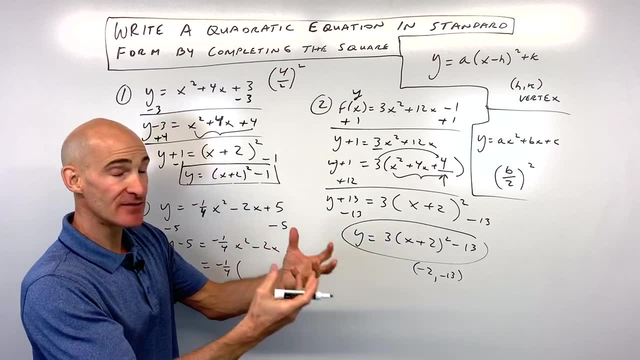 So now we have negative 1 fourth, x squared minus 2x. I'm going to factor out the negative 1 fourth, Okay. now here's the thing. When you factor out okay something, it's like dividing it out, right. 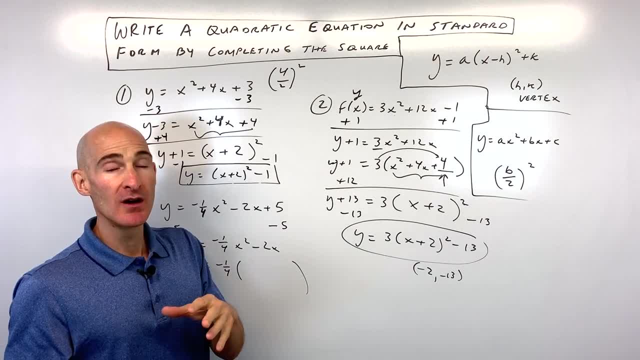 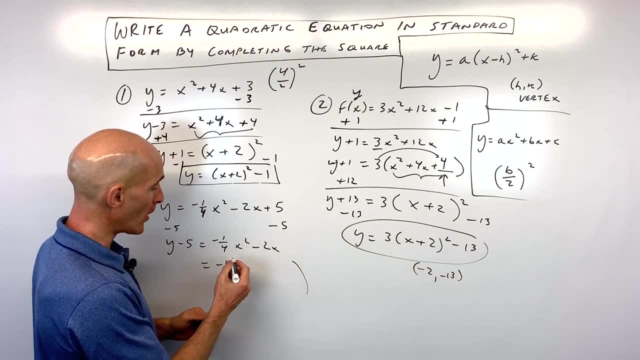 And so what you have to do on the inside of the parentheses here is you have to multiply by the reciprocal. okay, So here, because I divided out negative 1, fourth, I'm going to multiply by negative 4, and so that's going to give me x squared. 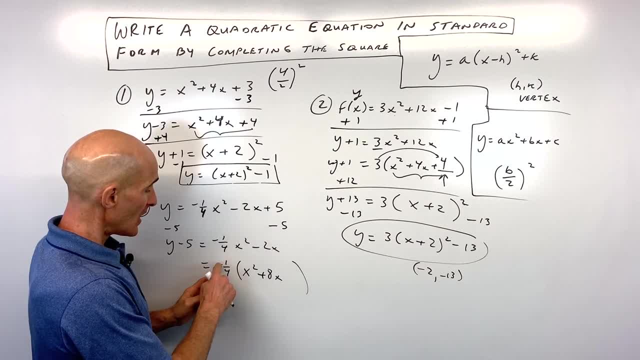 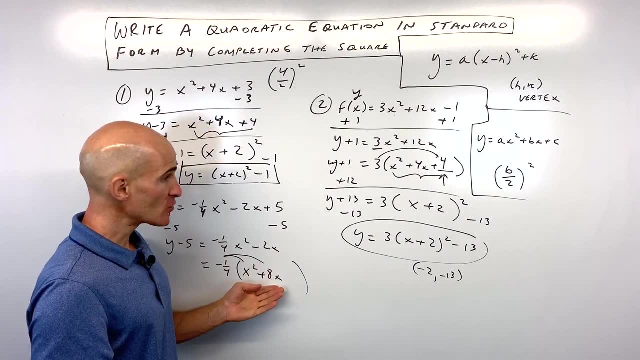 Plus 8x. Now, if you want to check your work, go ahead and distribute the negative 1 fourth in. You see that gives us back negative 1 fourth x squared. It also gives us back negative 2x. Here's where we complete the square b divided by 2 squared. 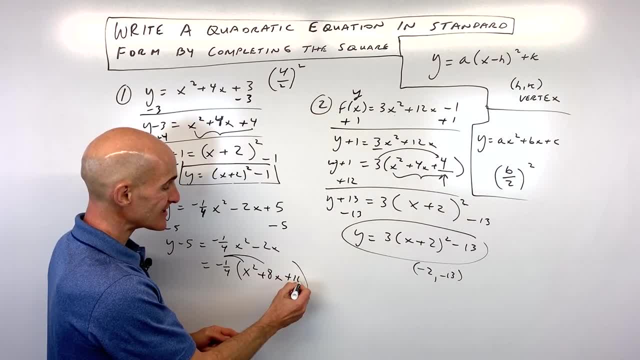 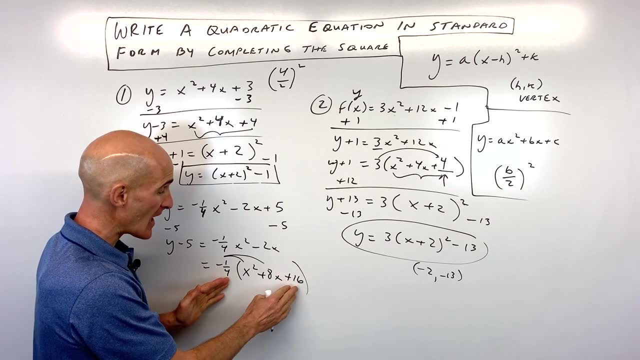 So 8 divided by 2 is 4, 4 squared is 16.. So do I add 16 to the left? No, because, remember, it's negative 1 fourth times 16.. I actually subtracted 4 from the right side because that's a negative 4, so what I'm going? 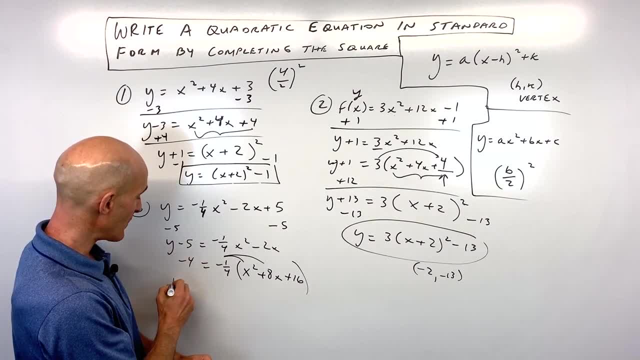 to do is: I'm going to subtract 4 from the left? Okay, so, I'm going to subtract 4 from the right? Okay, so, I'm going to subtract 4 from the left. I'm going to subtract 4 from the left side as well, to keep this balanced. 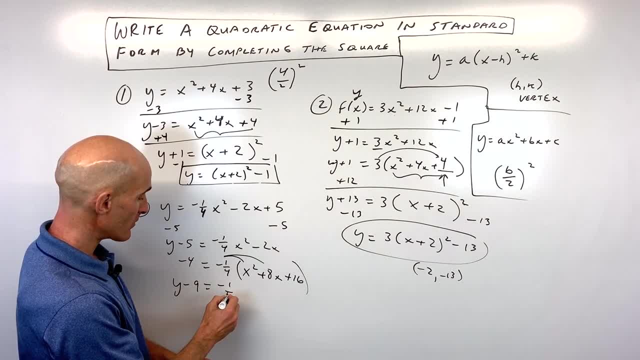 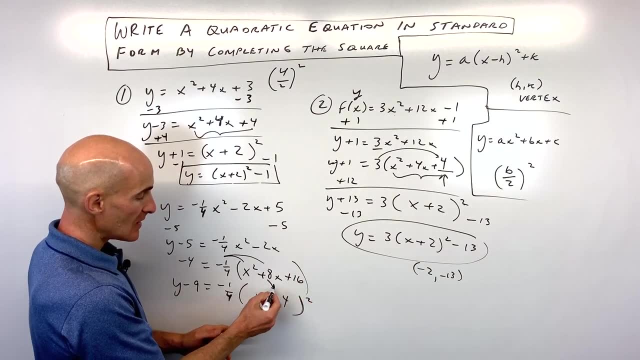 So we have y minus 9 equals negative 1. fourth, and now I'm just going to factor this: It's going to be x plus 4, the quantity squared, Remember, it's half of this b value. If it was minus 8x, I would write minus 4..